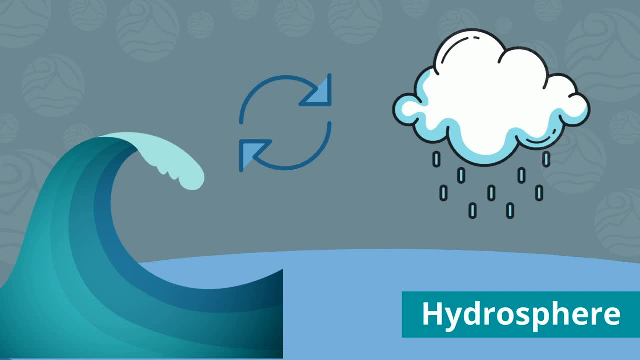 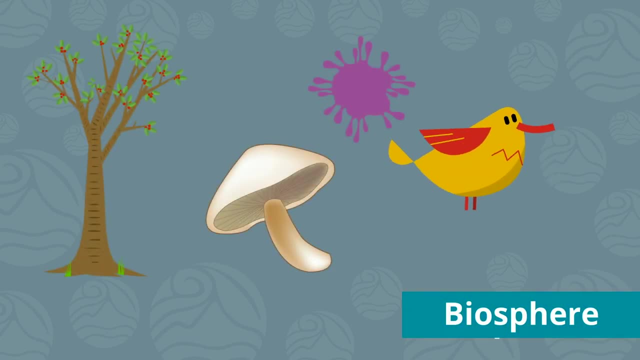 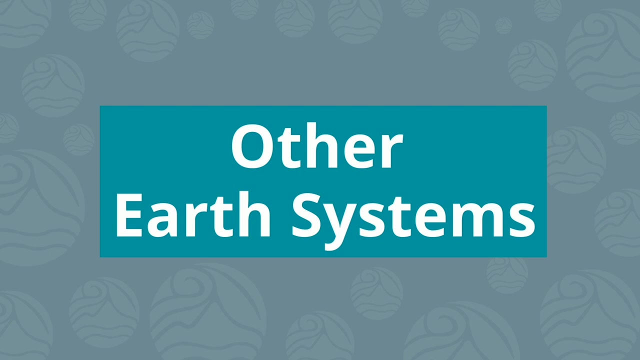 across the globe and how it all moves through the water cycle. The biosphere is made up of all life on earth. It includes plants, animals, fungi, bacteria and all the interactions between them, like symbiosis and predation. In addition to those main, four other earth 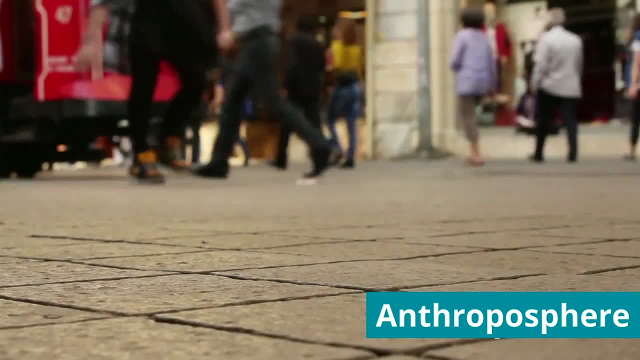 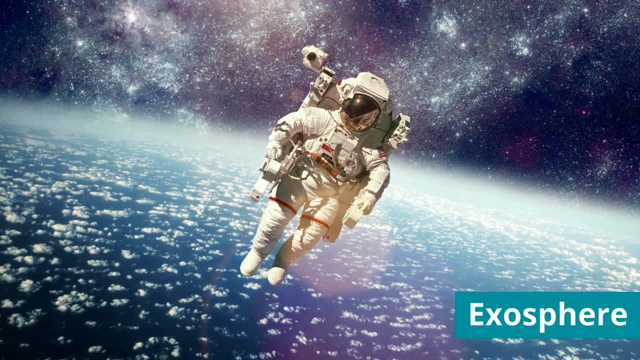 systems include the anthroposphere, human interactions, the magnetosphere, everything to do with the earth's magnetic field- and the atmosphere. The earth's atmosphere is composed of the geosphere and the exosphere, everything outside our planet like the solar system and beyond. 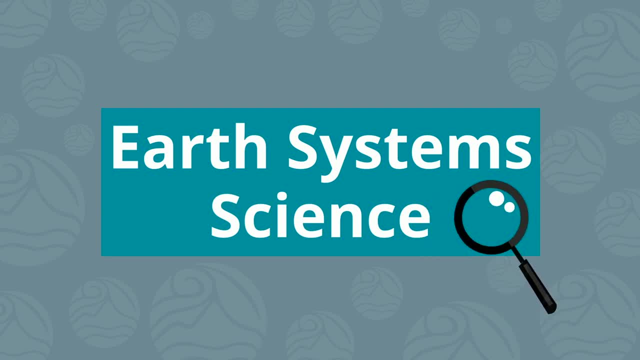 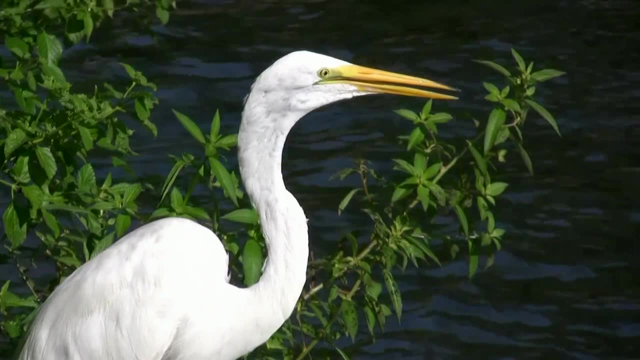 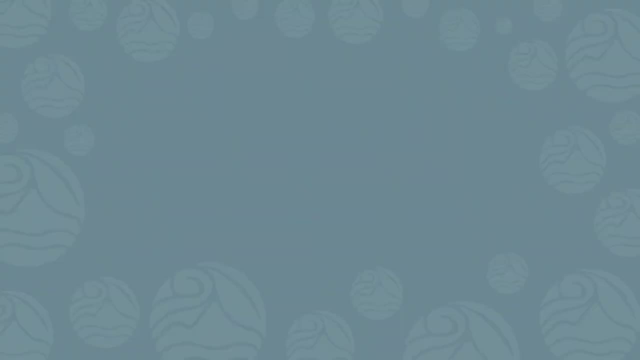 Earth system science is the study of all of these different spheres and how they interact. For a long time, scientists had studied things like air, water, land and life separately, But earth system scientists combined these different areas of study to understand earth as a whole, Just like how each ingredient of a pizza is tasty on its own when combined. 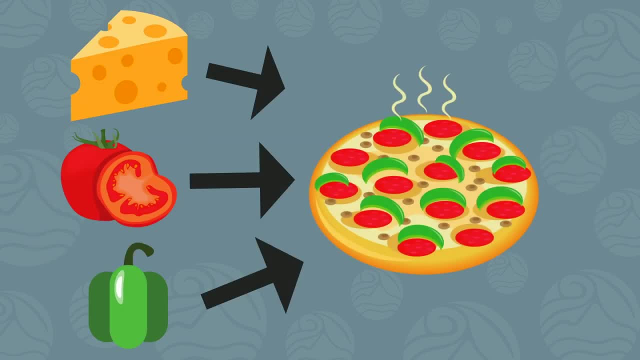 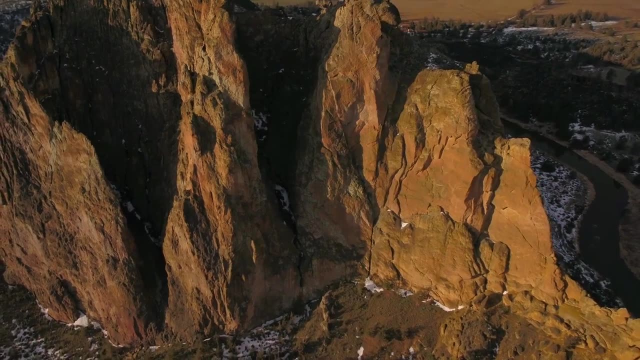 they offer a different taste. When combined, they offer a different taste. When combined, they offer a whole new flavor. perspective: Earth system science draws upon the fields of ecology, biology, geology or earth science, meteorology, chemistry, oceanography, physics and more to make sense of how our planet's 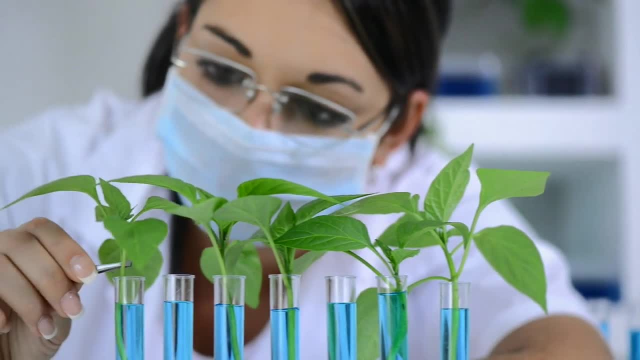 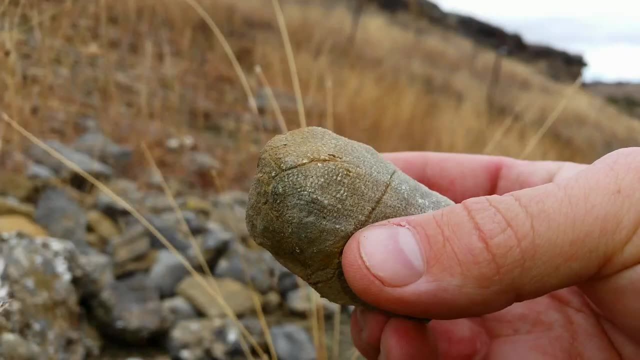 different systems work together. That's why this type of science is often called interdisciplinary, made up of many different scientific disciplines. Earth system science is important because it helps us understand how the earth's water systems work and how they Idierologia e Electricity. today, there's a community that 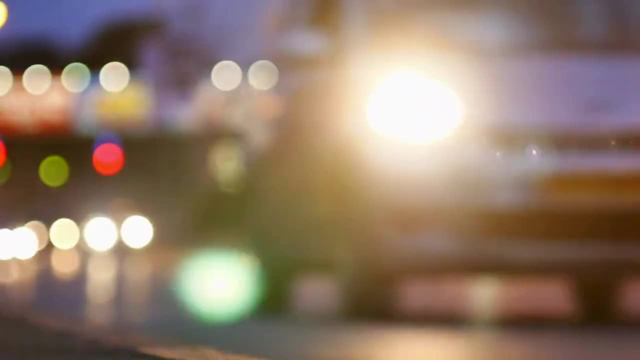 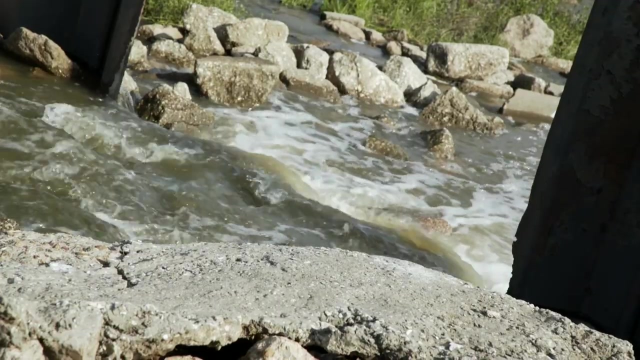 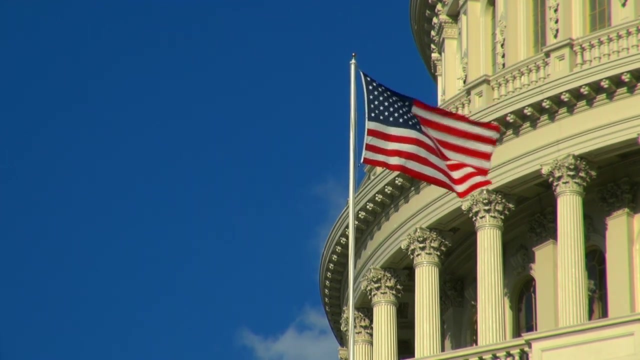 made what it's like now and how it will change in the future. Finally, studying how humans affect one Earth system and how that in turn affects others can help us make informed decisions about the policies and actions needed to preserve the health of our planet. Let's take a look at what an Earth system scientist 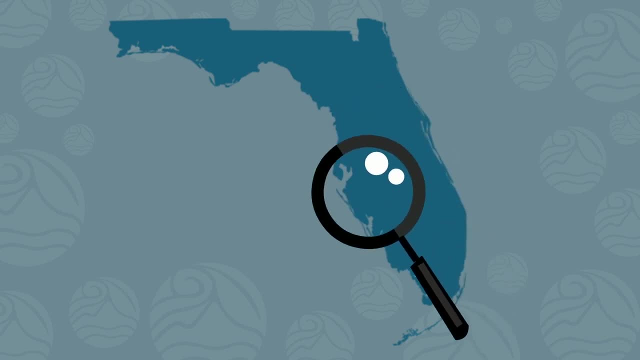 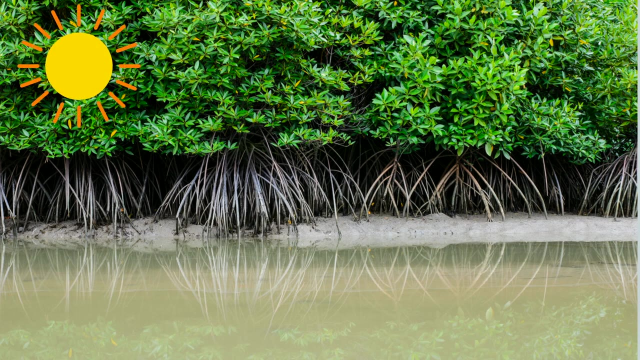 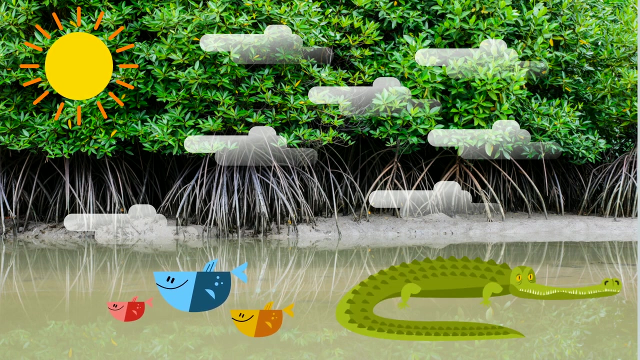 might think about when studying a Florida habitat. Consider a classic type of Florida ecosystem: mangrove, swamp wetland. Using energy from the Sun, mangroves and other plants produce oxygen that animals like fish, snails, birds, gators and more must breathe in order to survive. The waste produced by